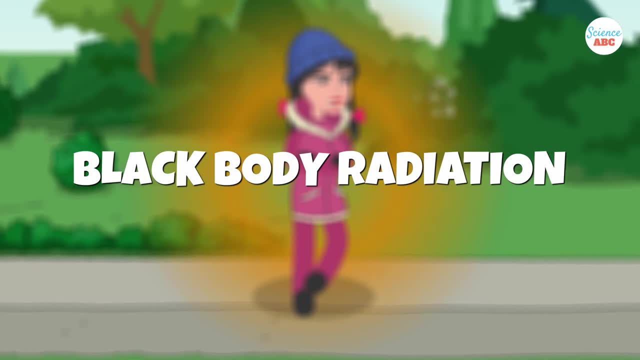 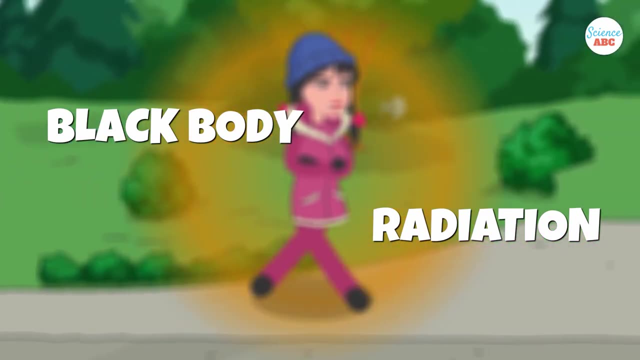 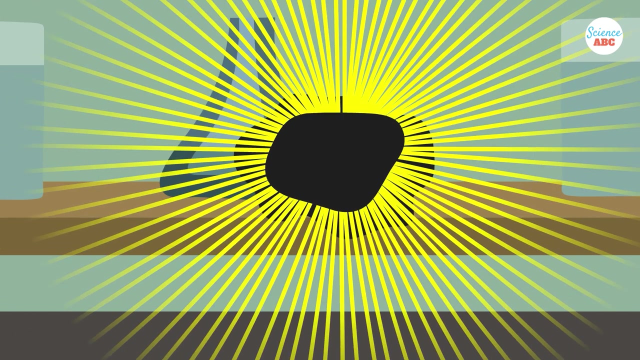 The principle of black body radiation is based on this concept. Now let's break down the term black body radiation to understand the idea a bit better. A black body is a theoretical or imaginary object that perfectly absorbs all incoming electromagnetic radiation and also emits radiation like heat and visible light. 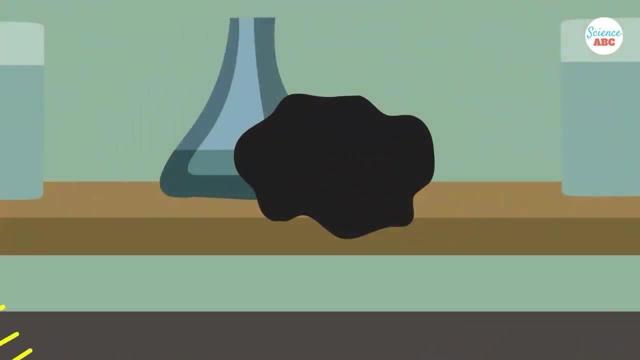 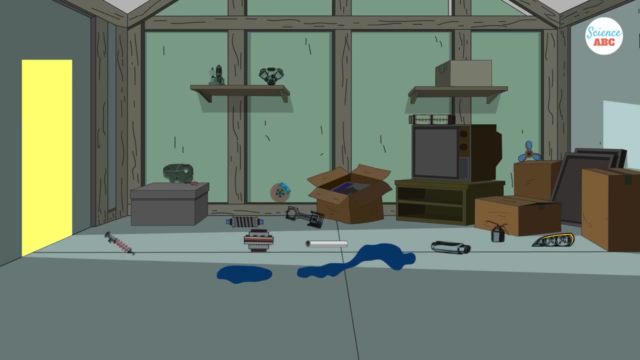 based on its temperature. A black body is considered theoretical because no object can be a perfect absorber of electromagnetic radiation. Think of it this way: When you heat an iron rod, it becomes extremely hot and its color changes to dull red, followed by bright red and black. When you heat an iron rod, it becomes extremely hot and its color changes to dull red, followed by bright red and black. When you heat an iron rod, it becomes extremely hot and its color changes to dull red, followed by bright red. 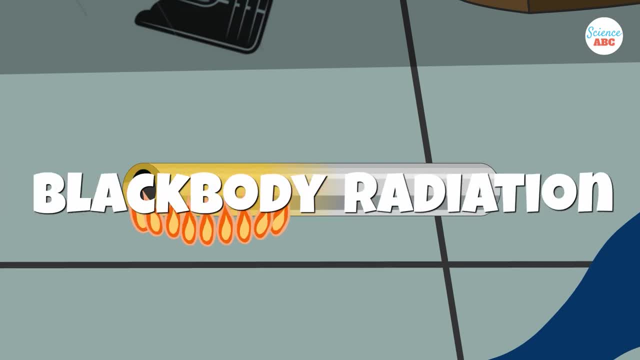 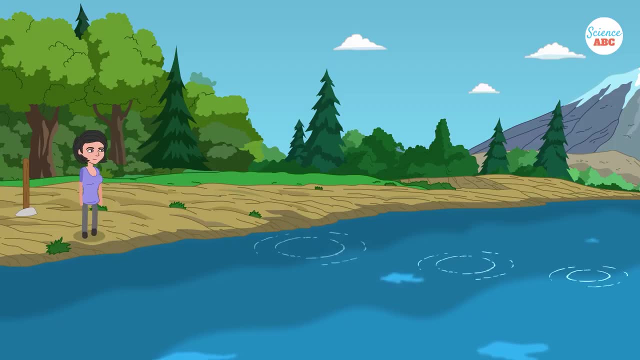 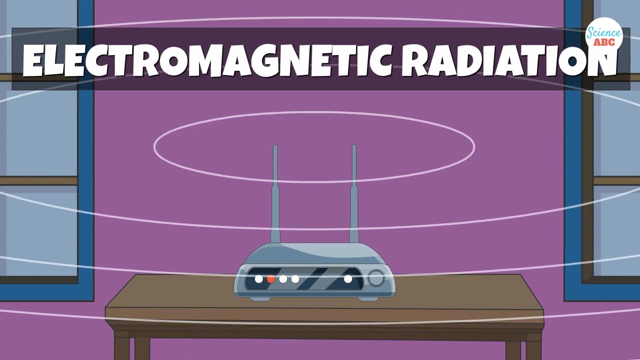 orange and then yellow. This is a good example of how black body radiation works. Imagine throwing a stone into a lake. It produces ripples that spread out in all directions. Electromagnetic radiation is somewhat similar, only, instead of being made of water, these waves 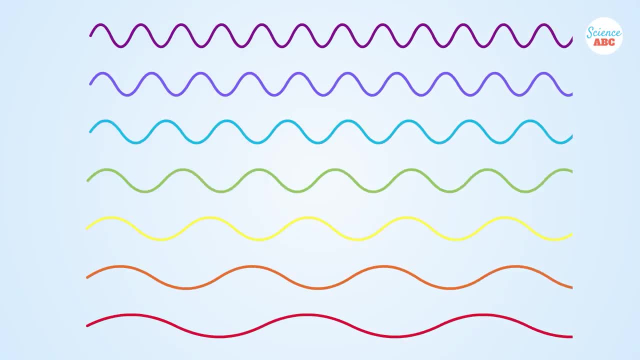 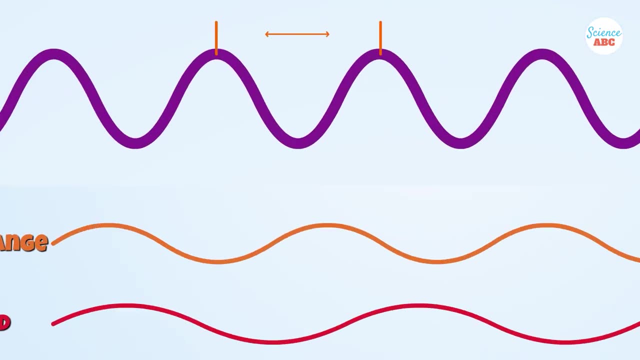 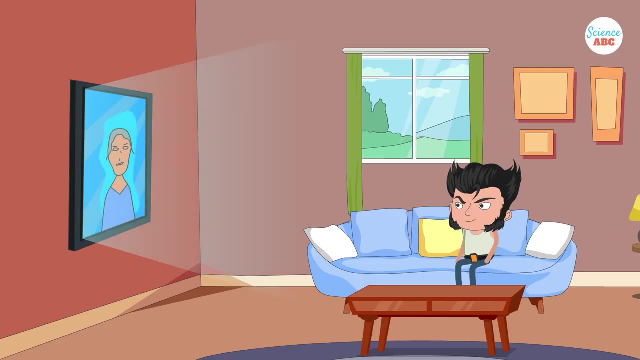 transport, energy. These waves are of different sizes or, in more technical terms, you'd say that these waves have different wavelengths. Some wavelengths are short while others are long, but each wavelength corresponds to a different form of energy, For example the light. 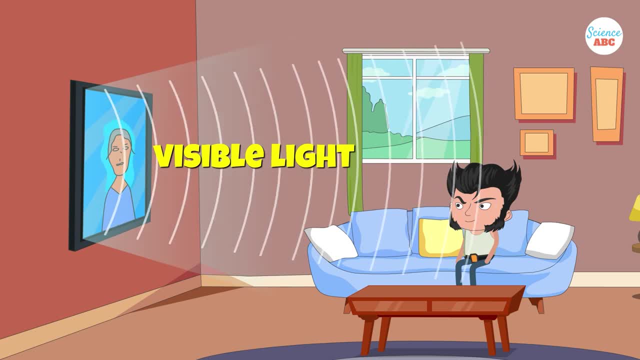 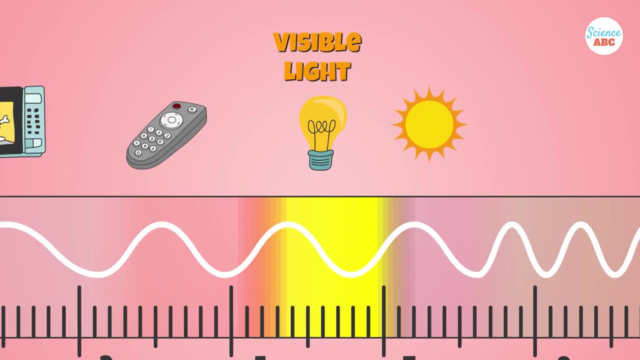 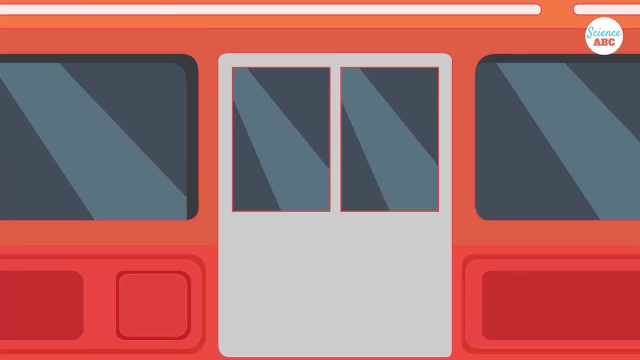 we see around us is also a type of electromagnetic wave, with wavelengths in the range of 380 to 700 nanometers. The human eye is able to see electromagnetic radiation that falls within this range, and therefore it's called visible light. Similarly, there is also electromagnetic 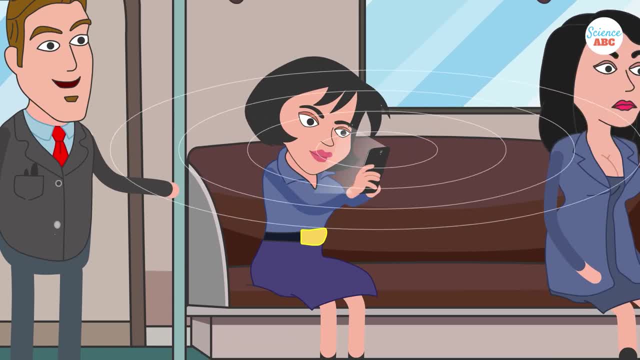 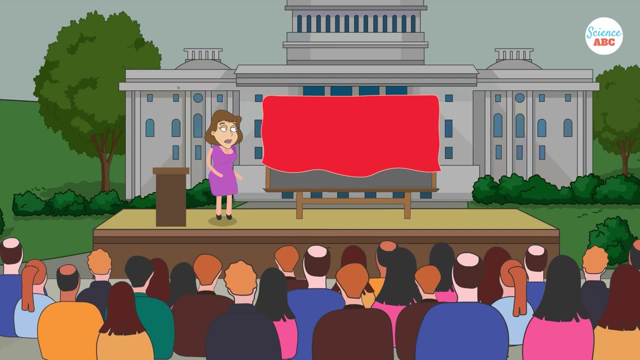 radiation that we cannot see, like radio waves with large wavelengths, which enable us to use smartphones and wifi. Another term you will often hear in correlation with black body radiation is the black body radiation curve. This is a simple graph that depicts the intensity of 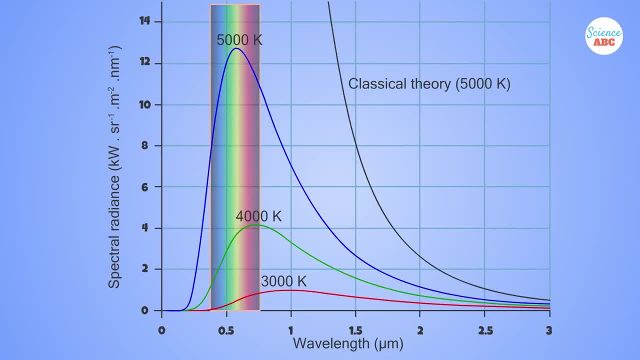 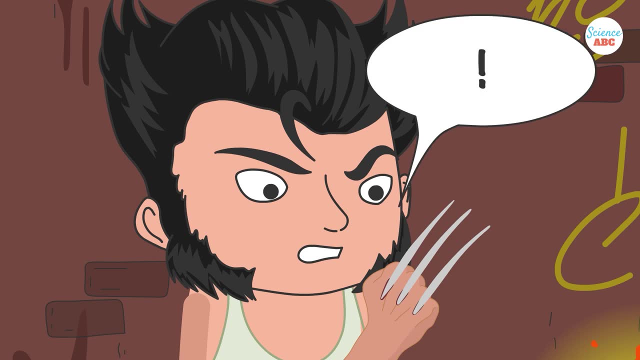 the emitted radiation from a black body on the vertical axis and the wavelengths of that radiation on the horizontal axis. Since the temperature of the black body is directly related to the intensity of its emitted radiation, you will notice that as the black body's temperature changes, the shape of the black body curve changes as well.